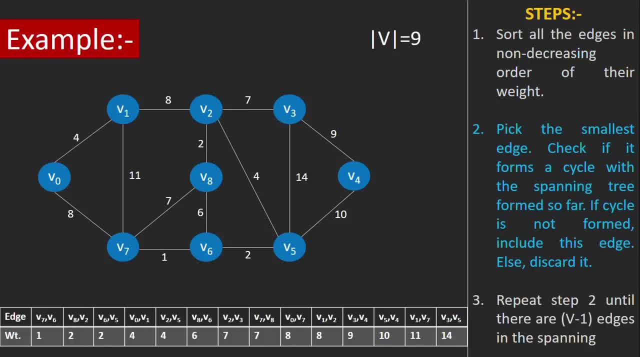 You can see that all the edges are written in the sorted order by their weights: V7, V6, being the smallest weighted edge, with weight 1, and V3, V5 being the maximum weighted edge, with weight 14.. Now let's move on to step 2.. Pick the smallest edge, V7, V6. Being the first edge. obviously, it does not form any cycle. 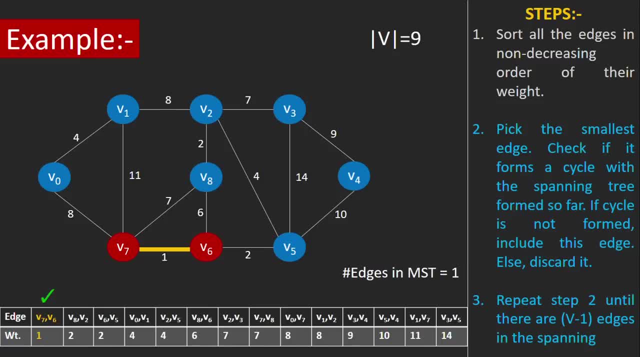 So this edge will definitely be a part of the minimum spanning tree. The edges represented by the yellow lines here are the ones that are part of the MST. Let's pick the next edge: V8, V2.. Again, it doesn't form any cycle, So it will be added to the MST. 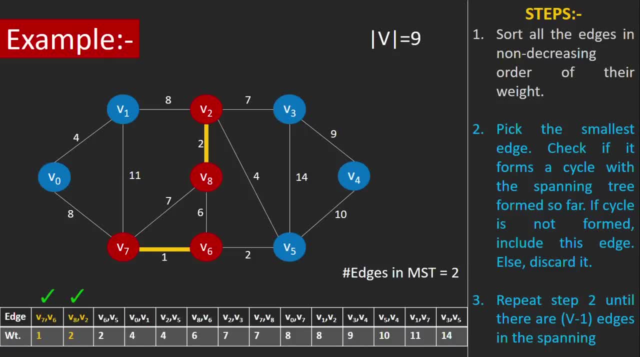 Next is V6, V5.. Again, no cycle being formed. Added to the MST. Now pick V0, V1.. Check for cycles. No cycle formed. Add this edge to the MST too. Next is V2, V5. 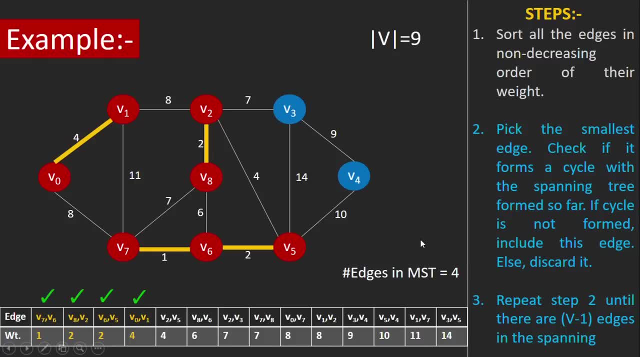 Again, adding this edge to the MST doesn't form any cycle. This edge will also be a part of the MST. Now let's look at V8, V6.. If we add this edge to the MST, it forms this cycle, as you can see here. 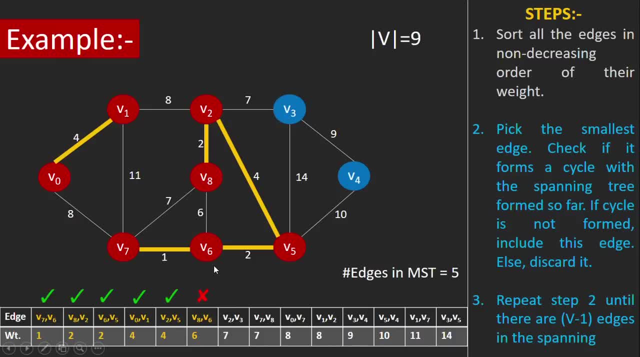 So this edge won't be a part of the MST. Now, adding V2, V3 to the MST doesn't lead to the formation of any cycles, So V2, V3 will also be an edge in the MST. Now V7, V8 can't be a part of the MST because adding this edge would form this big cycle. 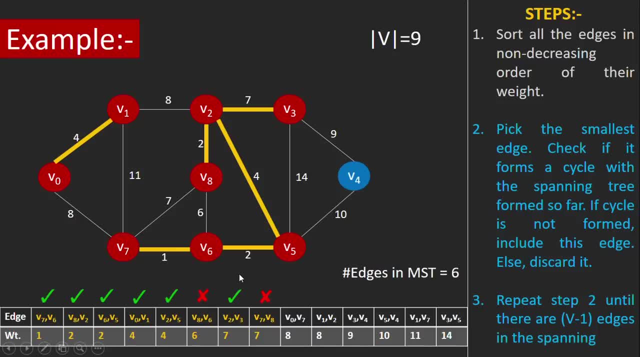 This one. Adding V0, V7 to the MST doesn't form any cycle, So it will be added to the minimum spanning tree too. Also, note that we are keeping a track of the number of edges in MST Because, according to the third step, we need to stop as soon as we have the number of edges in the MST. 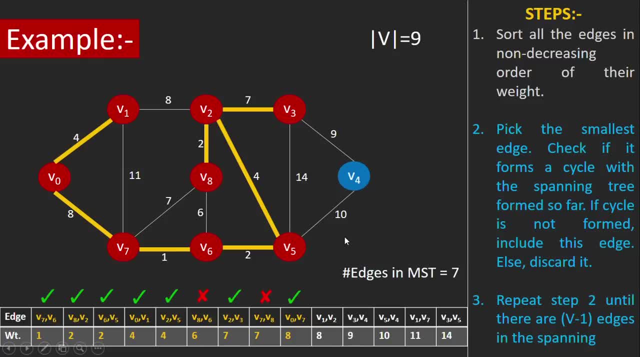 So we have V-1 edges, which is 8 in this case. Now let's try and add V1, V2.. Note that a cycle is being formed here, So V1, V2 won't be in the MST too. 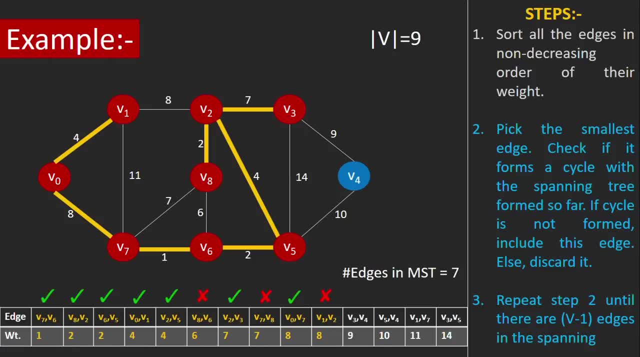 Next is V3, V4.. Adding V3, V4 doesn't form any cycle, So add this edge to the MST. Note that we have now 8 edges in our minimum spanning tree, So we have reached the terminating condition. Thus we have successfully obtained the minimum spanning tree of the given graph.